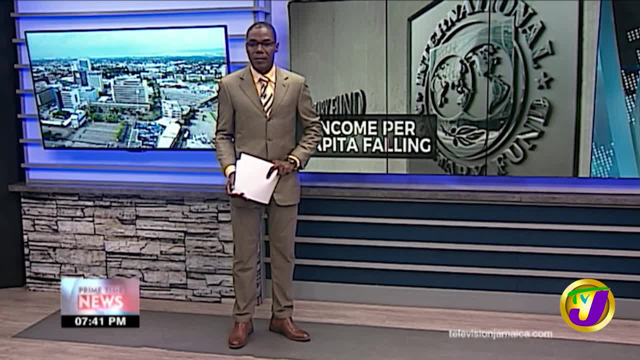 Welcome back. It's time now for the business day. The International Monetary Fund IMF disclosed today that income per capita in developing countries is likely to get worse before things get better. The IMF managing director was speaking ahead of the organization's spring meetings, which starts on Monday. Andrew Laidley has the report. 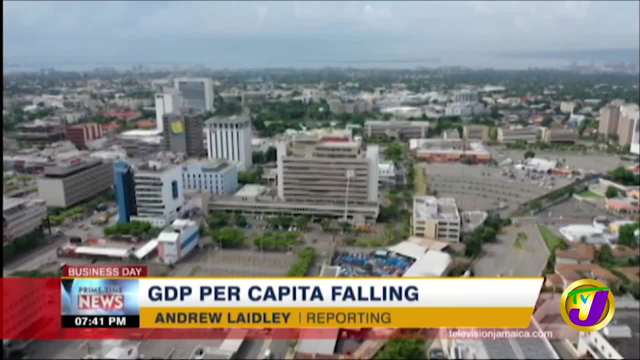 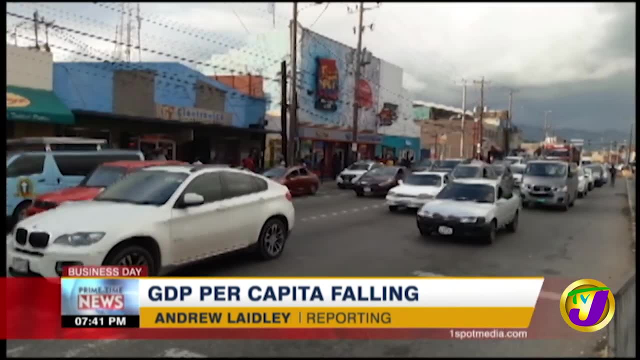 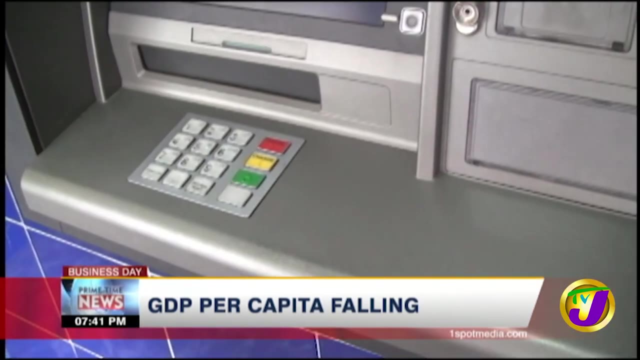 With lower domestic production and a higher jobless rate. Jamaica's GDP per capita has fallen since the start of the COVID-19 pandemic. This amid a projected economic contraction of about 10 to 12 percent for the 2020-2021 financial year. In short, 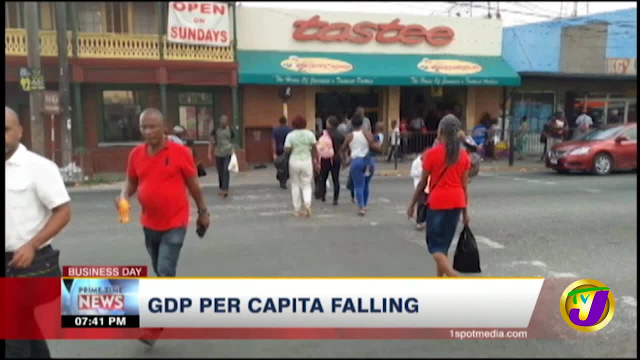 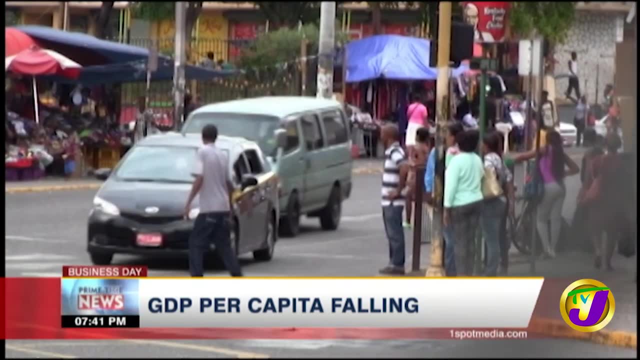 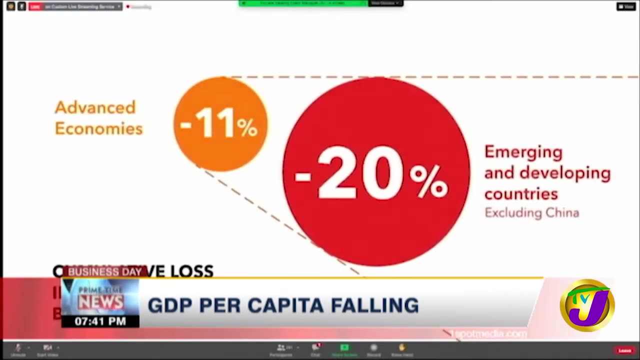 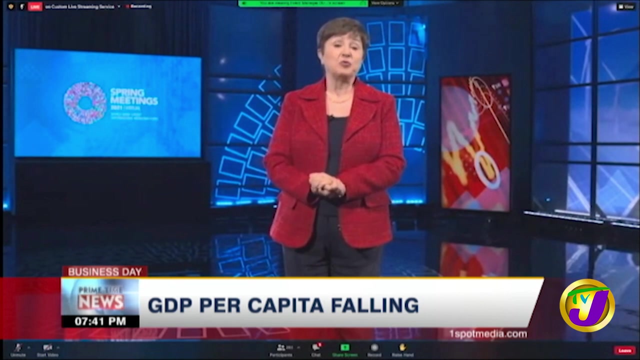 the average earning for Jamaicans has decreased, IMF managing director Kristalina Georgieva now highlighting that the income decline is likely to continue into next year. In developing economies, excluding China, the loss will be much worse, at 20 percent, Cutting one-fifth of what is already a much smaller per capita income than in richer countries. 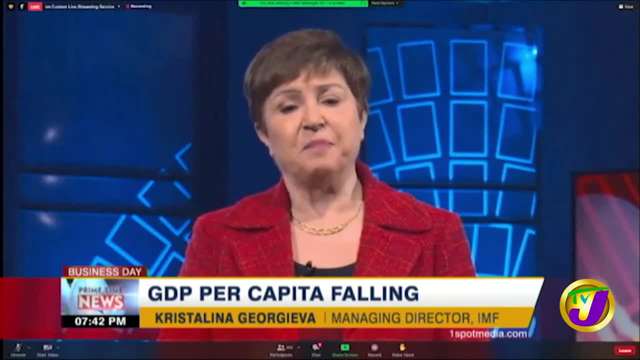 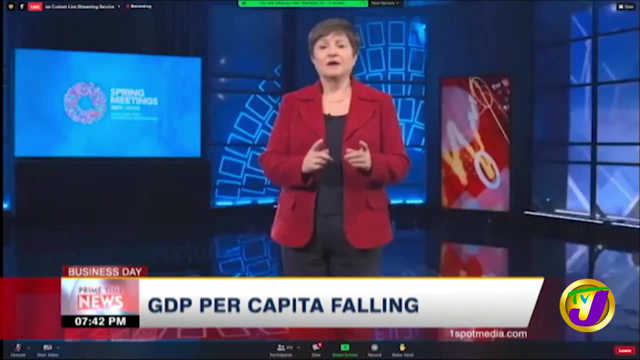 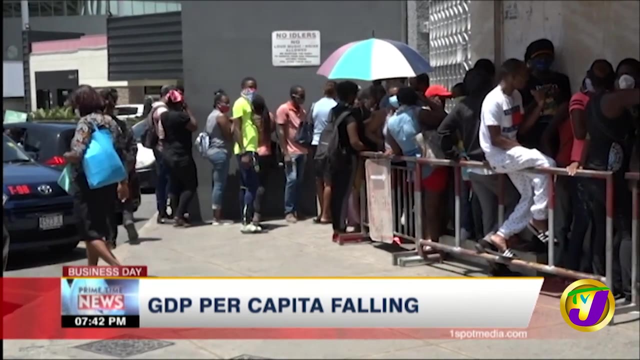 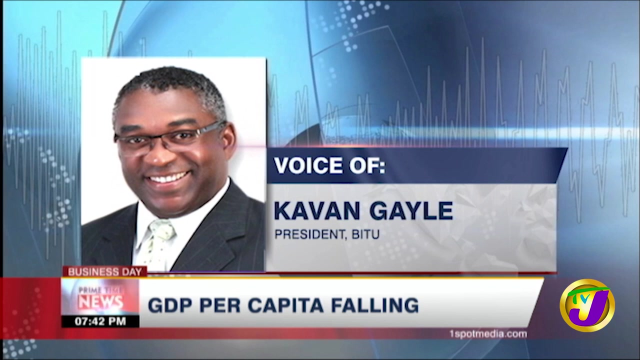 This loss of income means millions of people will face destitution, homelessness and hunger. President of the Bustaman to Industrial Trade Union, Senator Kavan Gale agrees: Despite measures of control and the emergencies of the vaccine, the economic unemployment consequences of COVID-19 is a crisis that is likely to exert. 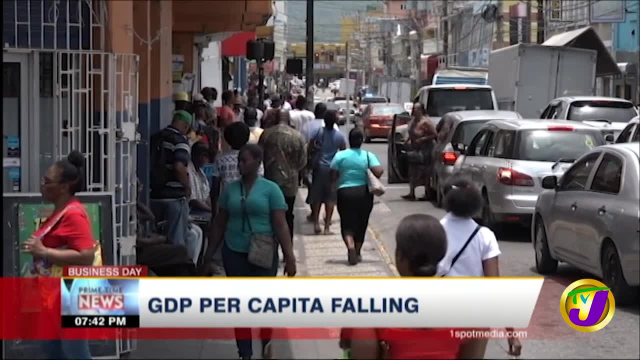 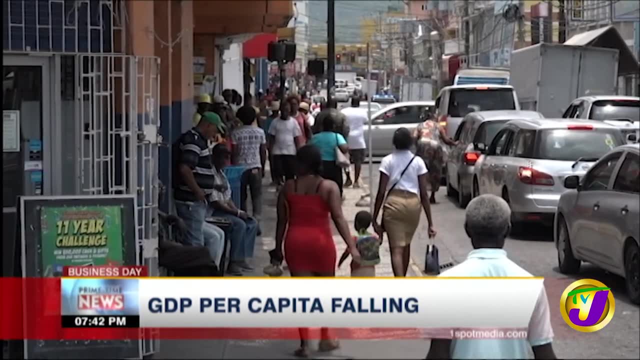 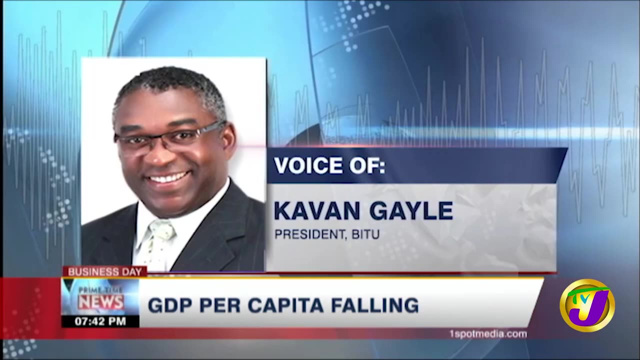 further downward pressure on wages in the near future. That's why the trade unionist is making this suggestion. We're going to need an improvement in wages that will lead and take into account the need for both income and aggregate demand to be supported for businesses to remain open. 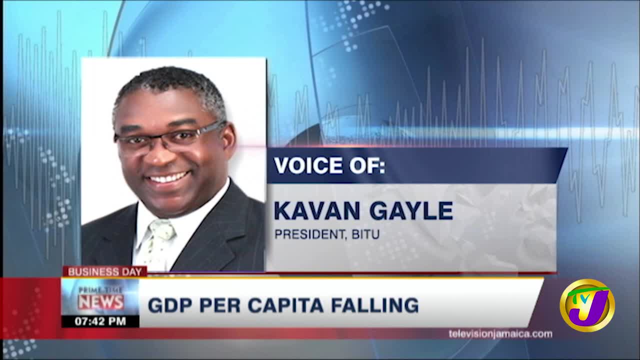 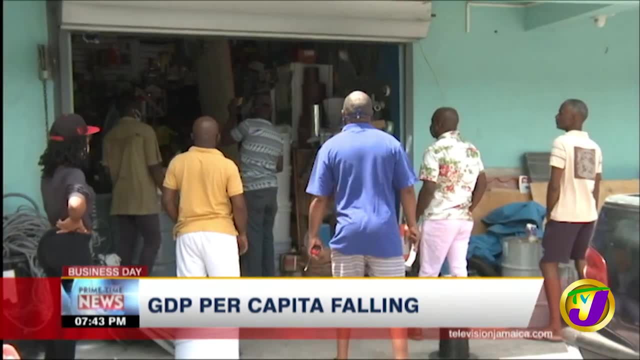 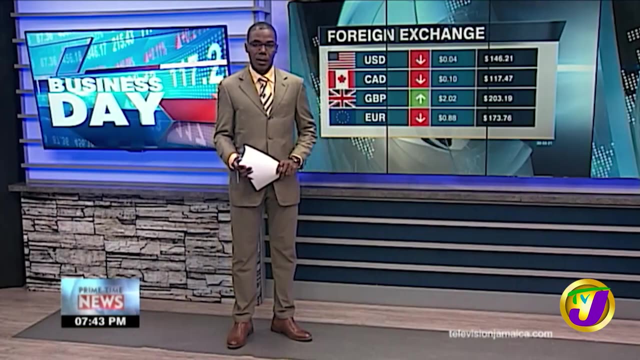 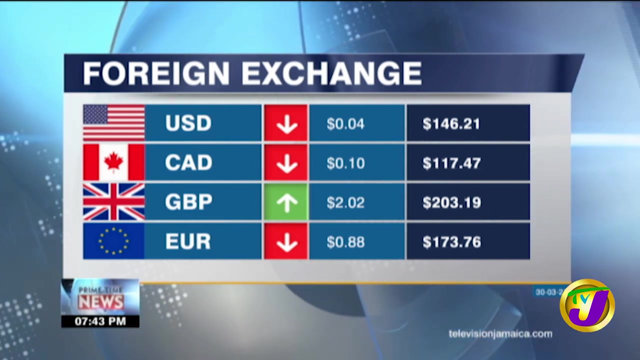 successful and viable. What it is going to require is that it's going to require constructive social dialogue between the state, the private sector, civil society and the trade union. That is going to be key. Andrew Lately TVJ News. The third wave of COVID-19 impacts in many areas of the world.